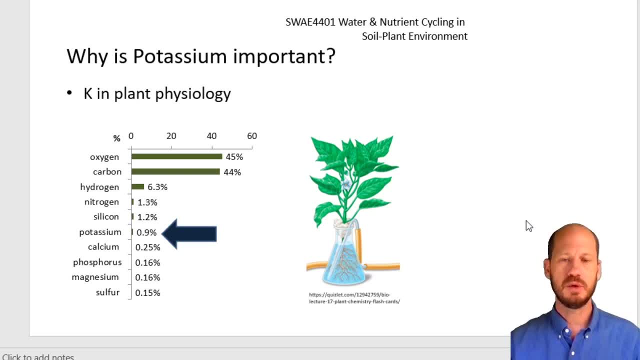 does not differ. we have the potassium is usually very high in concentration in plant tissues. one of the things that we have to keep in mind is that in the case of potassium, the plant concentration of this element is very variable. you can have that if you have deficiency, you have a low concentration of potassium. 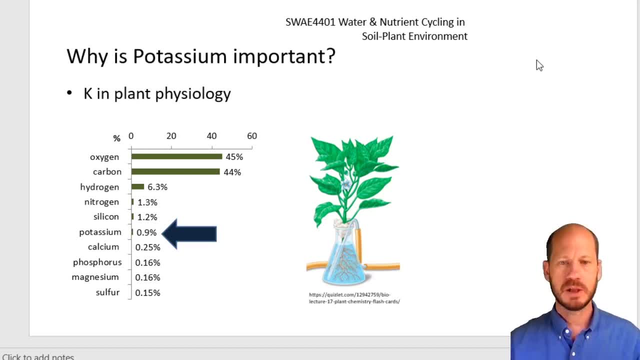 and when you have excess potassium on the soil, the plants will over accumulate this, so you might have the. potassium is very, very abundant in plant tissues and it doesn't mean that is the main nutrient or the one with the main roles in the plant, but it does have very important roles. yeah, one of the things. 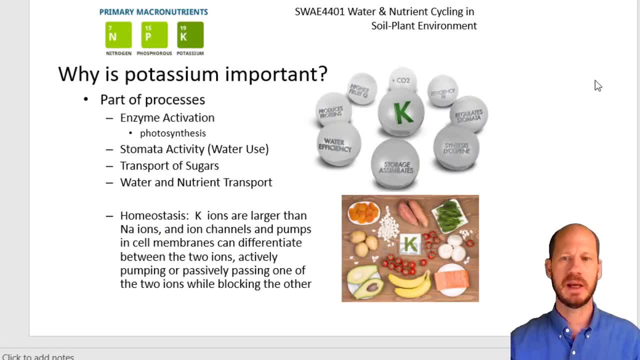 that we have considering from potassium in plants is that potassium usually- not ever- is part of any molecules in in in plants. you know it does not. it's not significant, but it is important to know that. it is important to know that it is not structural to any plant molecules, potassium inside the plant tissues as it. 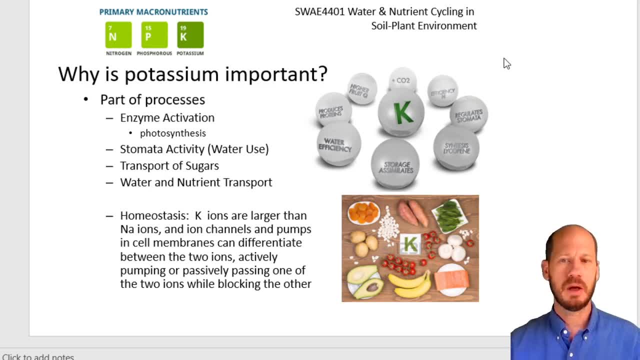 is in the soil, it's always in the ionic form, so it all its roles. it's regarding the its presence in ionic form, so it the open enclosure of stomata, regulated heavily by potassium, or, and therefore photosynthesis, gas exchange water used by the plant, new tissue growth. this all dependent on potassium- potassium. 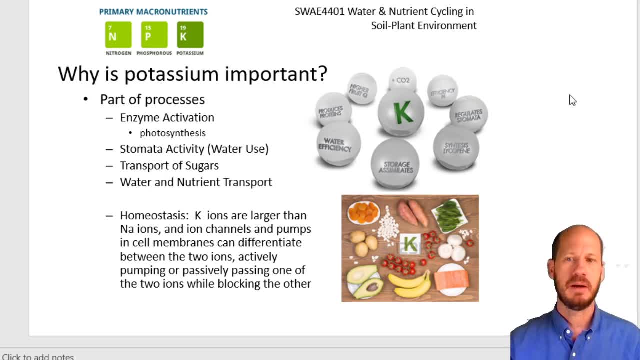 because of its role, as in the in its ionic form it it's a counter ion for most anions, organic anions that a plant produces, so such a citric acid, oxalic acid and etc. potassium together with calcium inside the plant tissue. they are the counter ions that equilibrate this anion. 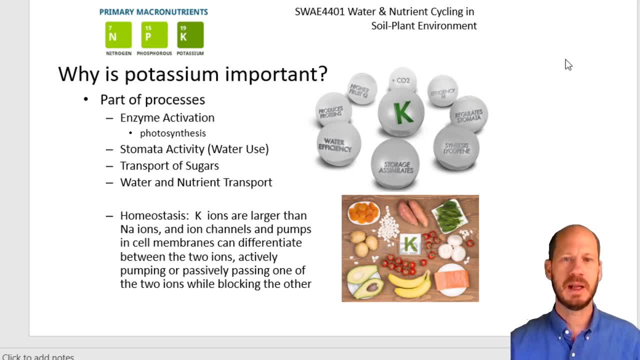 Potassium is also very important in enzyme activation and transport of sugars and in some climate, cold climates- potassium is very important for the resistance to cold. so potassium fertilizer application is very important for plant physiology. if you don't have sufficiency of potassium you will have serious problem with the water use usage, photosynthesis- the enzymes will be less. 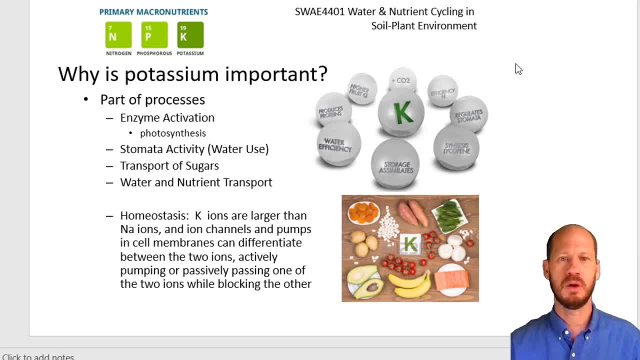 active. you know, in the cells there's a big role of in potassium on conditioning that ionic strength needed for some enzymes should be on the proper folding to perform its catalysis inside the plant tissues. and in general you can say that potassium is always regulating the 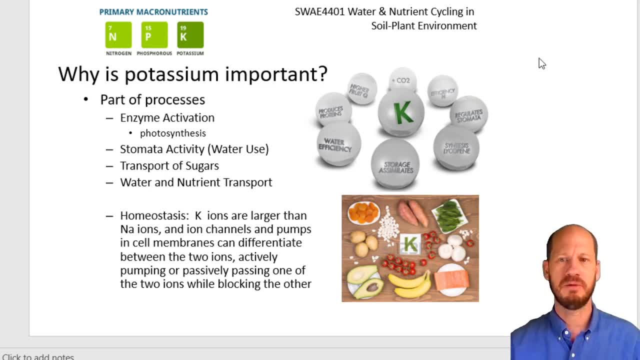 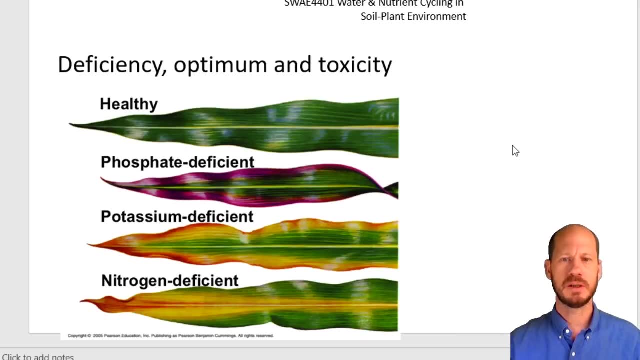 these homeostasis in the plant tissues, this equilibrium of ions inside the plant tissues. when you don't have potassium, you will always identify this clearly by intravenous chlorosis. yeah, if you the yellowing, but the stripy yellow features that you have the in the in the leaves and also because of less growth. 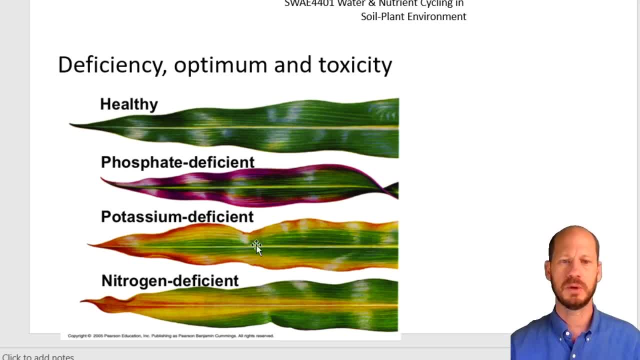 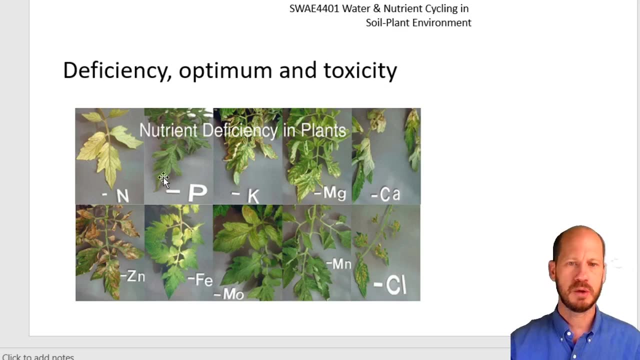 of the plants. also, you're going to be have a lot less growth without with potassium. but this striping intravenous chlorosis is what you will see very often as a potassium deficiency. here again in tomatoes, how it looks like comparing to what you see from phosphorus. phosphorus there's no yellowing at all. nitrogen is. 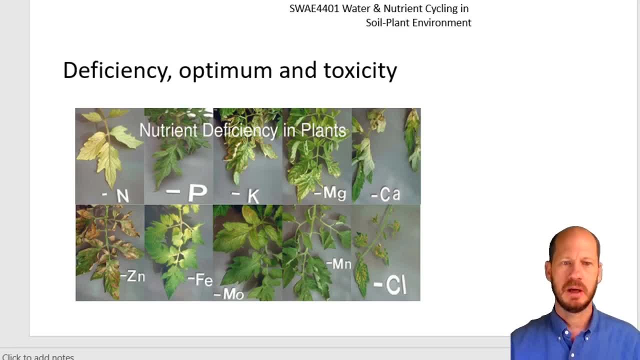 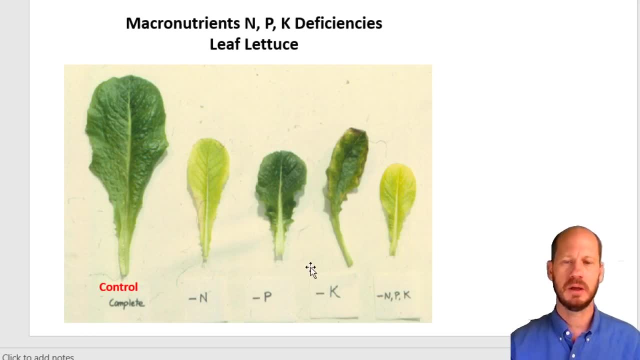 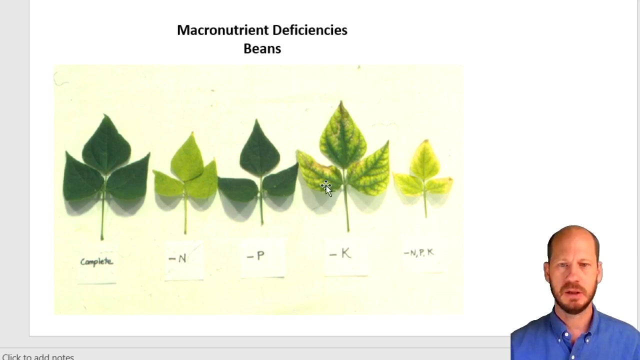 only yellowing. but potassium has these patterns in the leaves you can see here in lettuce. you can see a little bit of burning also on the external side of the leaves. with with less potassium, for beans also, this is what I was referring to: this kind of patchy patterns that you see on leaves. this is very 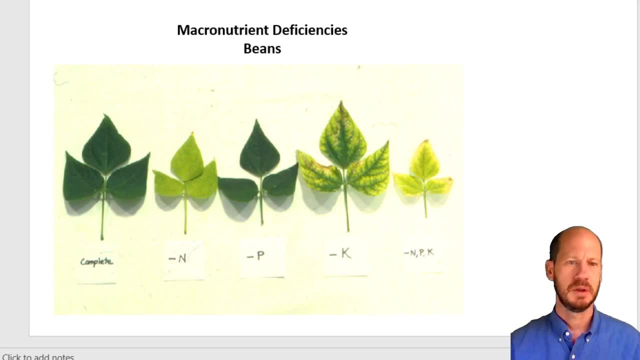 characteristic for potassium? yeah, very characteristic for potassium, and because plants need potassium in high amounts, usually, when you see this pattern, it's a good indication that you might have potassium potassium deficiency. so for the biogeochemical sign, Welcome to my channel and welcome to my English class on Before Господь заработок. 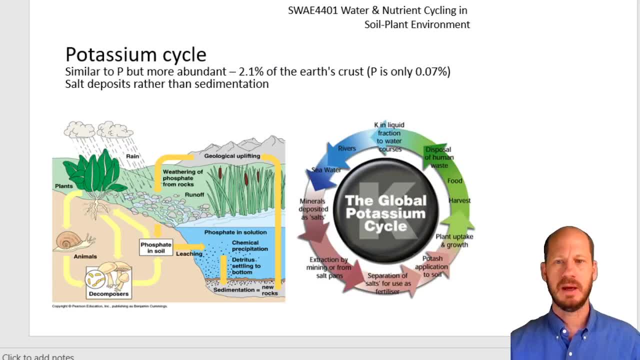 So for the biogeochemical sign of potassium deficiency, there is a question that I would like to see. we have to keep in mind that in this perspective- not in our perspectives, but in this perspective- it's the potassium cycle. it's more similar to what the 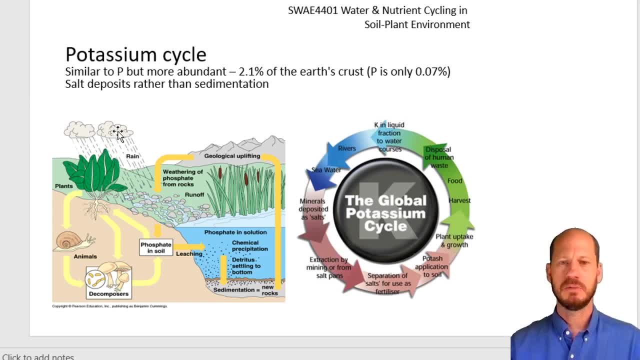 phosphorous cycle is. you know you will have that. the potassium cycle has very little to do with atmosphere. you can have some dust containing potassium, but mostly the the. the potassium is moving through the earth systems, through the water and then, by geological uplifting, you will have this formation of the. 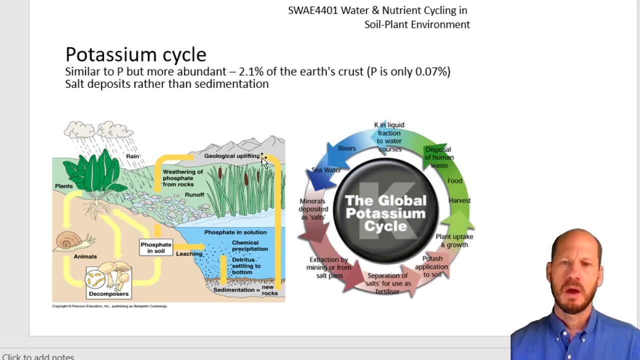 feldspars and potassium rocks also. but the the case cycle is it does not cycle through the atmosphere, it's the. the decomposition of the rocks is the main source for the soil environments. from the soil this potassium is lost to waters and then again going through the biogeochemical cycle of terrestrial 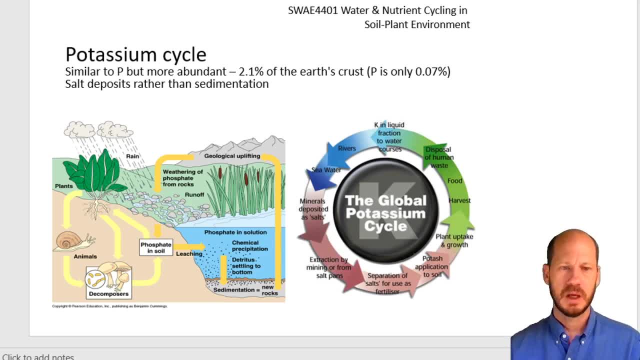 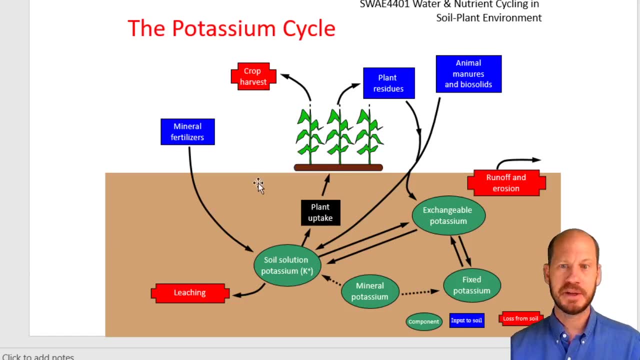 systems to the weathering of these rocks. if you focus a little bit more in the soil environment, you will have that the the main in natural ecosystems, the main source of potassium is the weathering of rocks. usually feldspars are very rich in potassium and if you have this feldspars as parent materials you will have high. 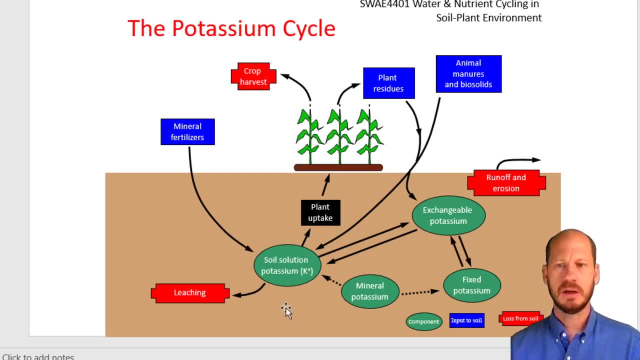 potassium soils. otherwise the mineral fertilizers are the main source of potassium for most soils. if you don't have potassium rich parent materials, then mineral fertilizers have to be the main source of this element for crops. you have that in soils. there are not many transformations. you will not find. 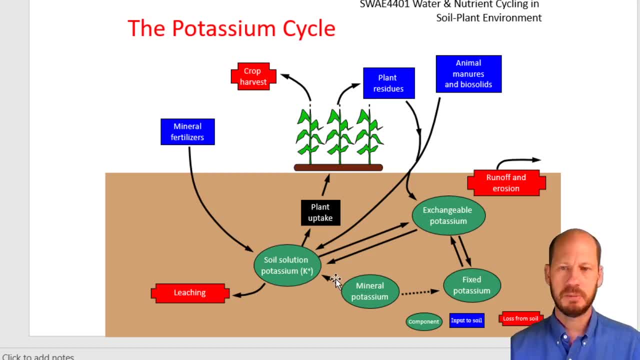 organic potassium or precipitated potassium in different ways. potassium can adsorb, but its adsorption is not so strong. also, what happens is there is some interaction between potassium and two to one clays, but it's not not heavily about surface adsorption, but it's more like the potassium can sneak in the 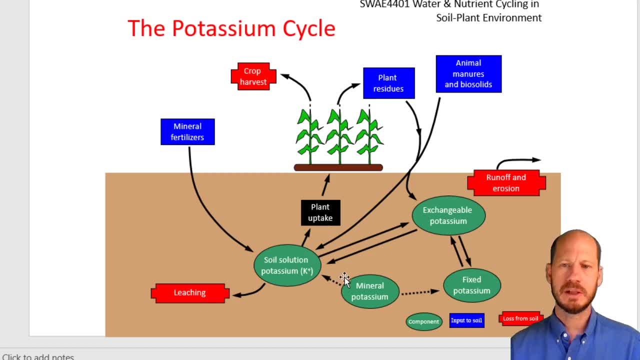 layers of this clays and you lose potassium from the crop, from this soil, mainly by leaching and runoff and erosion. also, you can lose a lot of potassium from the soil by crop exports because the plants have this ability of over accumulating potassium and if you have a high potassium in the soil the plants will take more potassium than they need in the 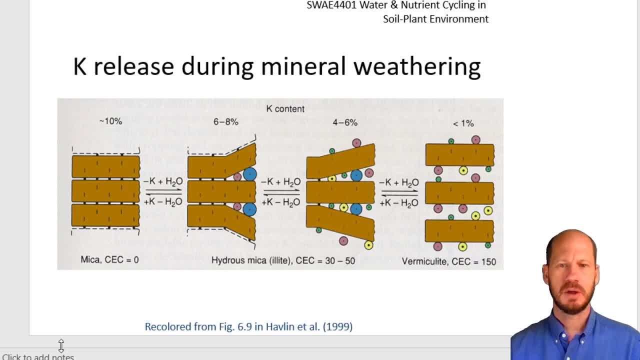 plant tissue. okay, so this is what I was talking about before. this is showing this ability of potassium to sneak in the, the interlayer of different clays, like montmorillonite, for example- all two to one clays and you will have the potassium will be being able to get inside. 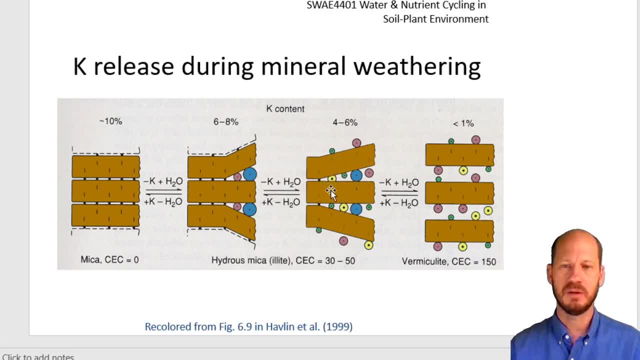 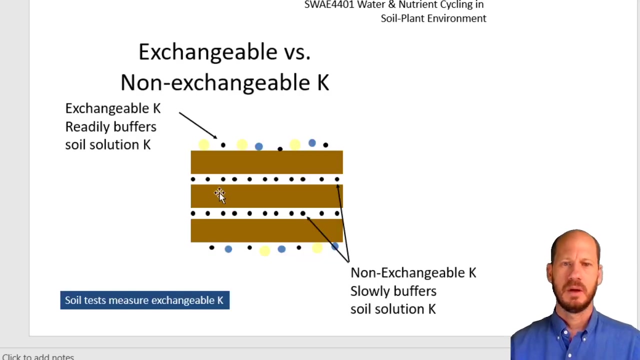 this, this, this layers of the, the sheets of the clays, and by doing that it will become unavailable for plants in. this behavior is highly dependent on the weather in and how moist the soil is in the. the seasonality of this, this fixation of potassium, is very heavy. you know, the seasonality of this fixation is very heavy. so the ones that 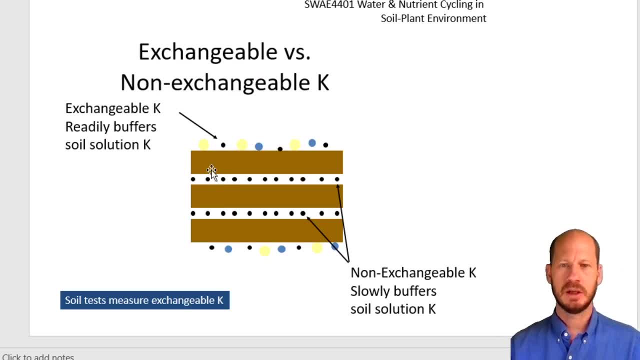 are in the surface of the clay outside can be exchanged. this is but the ones that are inside the clay particles. they are not immediately available to plants and the release is very slow. so there is some fixation of potassium, but its mechanism is very different from what. what the fixation of phosphorus is. you know, fixation of phosphorus is mainly 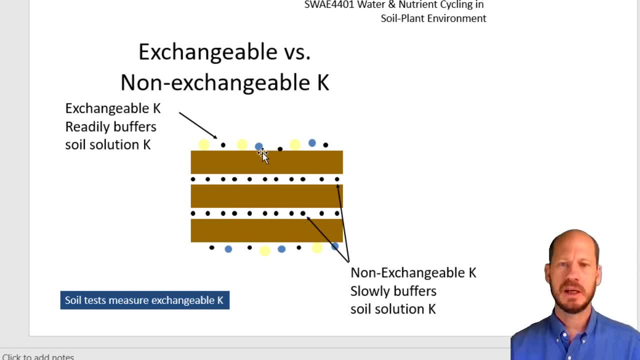 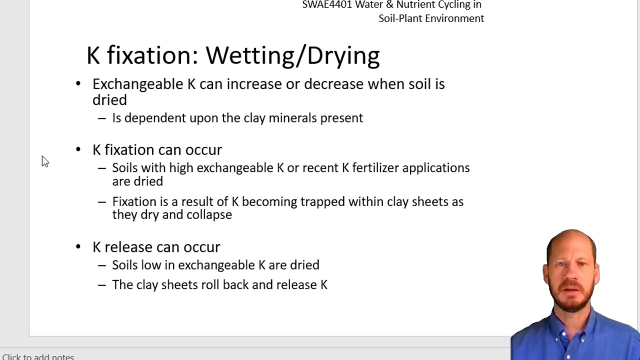 adsorption, precipitation and immobilization in organic molecules, whereas potassium is always associated with this two-to-one clays and this ability of the potassium to be locked inside this, the sheets and layers of this two-to-one clays clays. so this fixation, as I was telling, is highly dependent on the wetting and 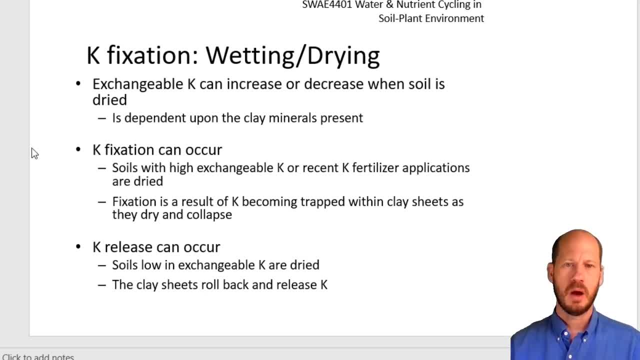 drying of the soils. so when you have that, the soils become very dry. you will tend to have some more fixation of this potassium. okay, it happens also when you don't have this 2 to 1 clays, you lose the ability of the soils to retain the. 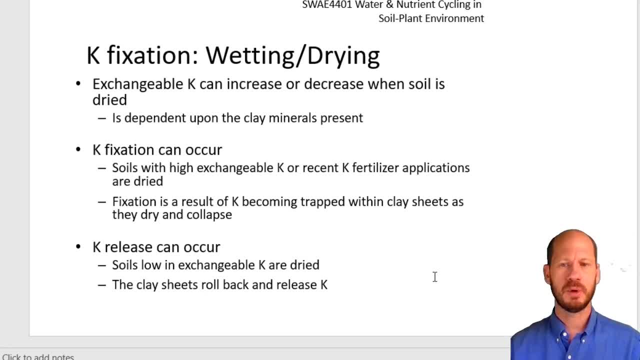 potassium and usually these soils will become very poor in potassium because of the potassium leaching. you know, because potassium is so soluble. when you have this 2 to 1 clays, you immobilize them in unavailable forms but in a sense you are also able to store some of this potassium for the next cycles. 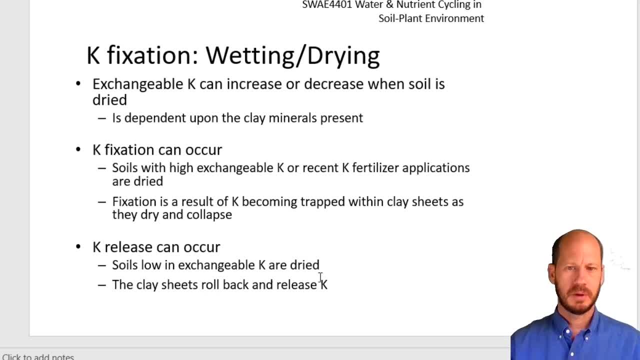 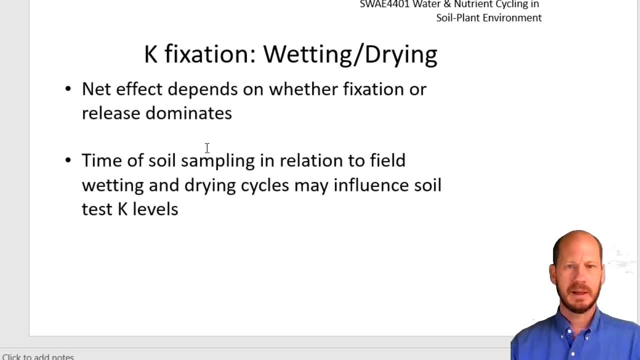 yeah, all right. so the net effect depends on whether you are in the cycle of drying or wetting, depending on the seasonality, and this is which one is dominating. depends on the season of the year, and so you might have a strong variation of the the soil test. 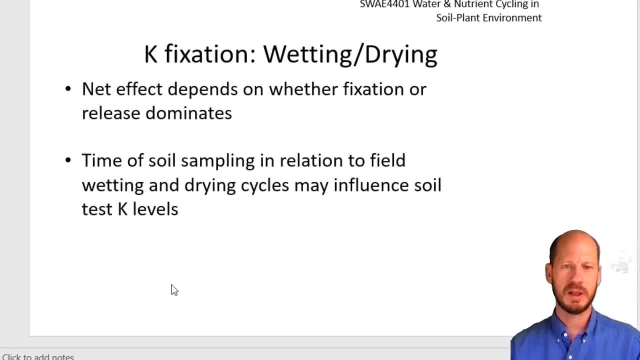 potassium throughout the year due to the wetting and drying of these soils. you will always think about the soil test potassium. you have to think about whether you are in the same time of the year and in the same weather conditions. are you doing after a rain event or are you doing in a dry spell? so you have to. 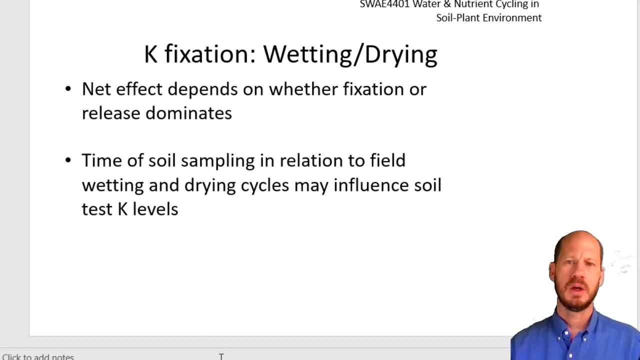 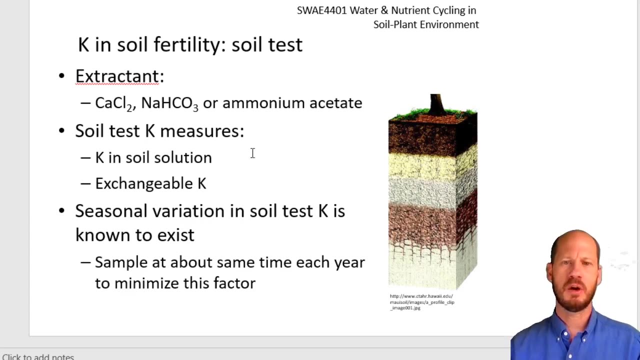 think about when you do this soil sampling for potassium. you have to think about the soil moisture to try to keep this a little bit more uniform, you know, to keep it uniform and less varying throughout the seasons. so you have different extractants for potassium, but these are always weak extractions and 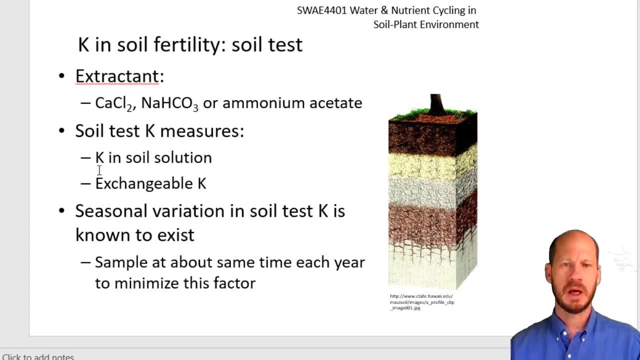 even though we're not using the advanced method of soil sampling to test these potential cesium nourishment. but also this is an example of UV radiation here. so we have a typical case here. we have UV radiation combined with firearm, and I will show you if I have this particular case. 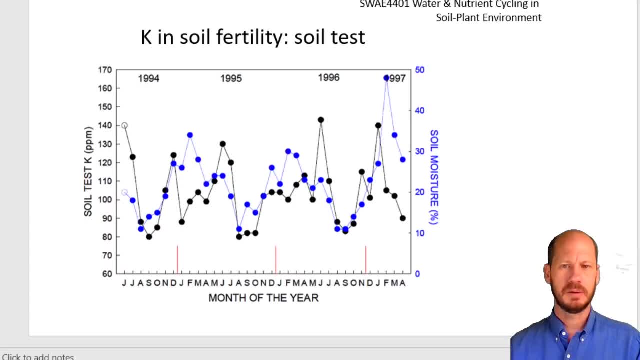 normally. but we have this case here and it is different to the previous case. usually the potential cesium is 1, 1 times higher than 1 where the pesticide is, and here is showing how it's happening. so you can see here that between 80 and 140 this is a very strong variation, almost a hundred percent. 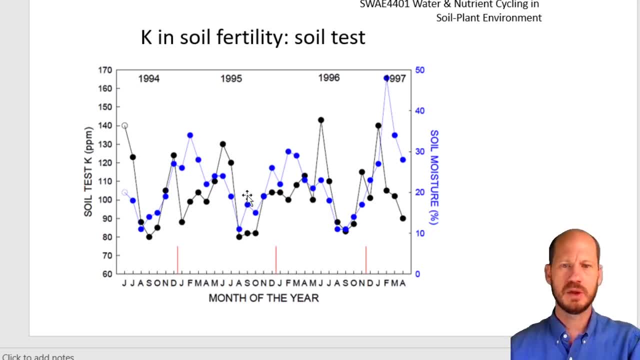 change and this is why you cannot trust too much the soil test potassium as a way of fertilizer recommendation. so it gives you a hint of if your potassium is in a sufficiency level. or let's say, if you measure 20, 30, 10 ppm, you for sure. 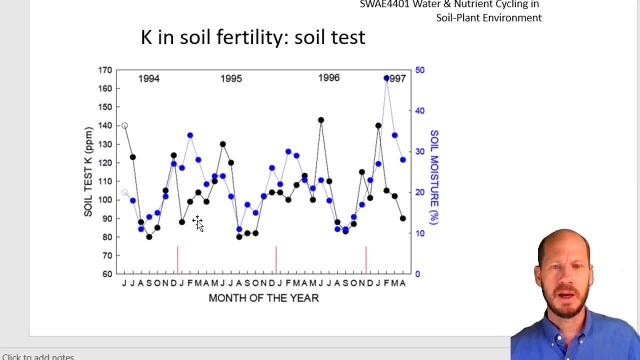 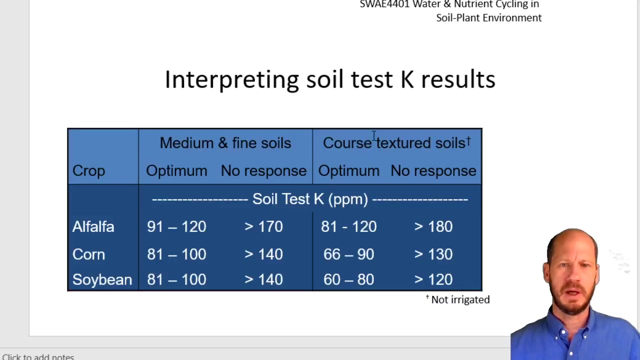 you have a potassium deficiency, but if you measure 90- 100, you might have deficiency or sufficiency. you for being on the safe side. you should be applying potassium when you measure on the low side of the bioavailable range. okay, all right. so how to interpret potassium results if you have something over 100? 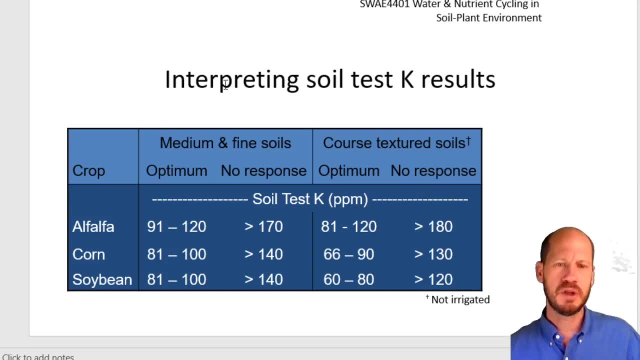 ppm. in general, you consider that you have sufficiency between 100 and up to 160, 170, 180. this is usually what you consider a sufficiency level. if you have over 180 usually is excessive. yeah, you usually is excessive. yeah, you will. you might find loads of. 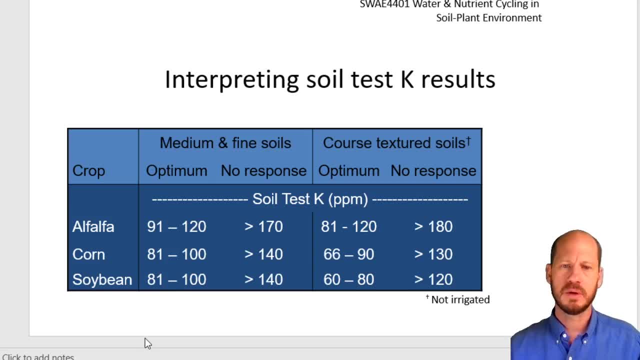 tables recommending this for different crops, but actually because the soil test is not very accurate, I would recommend not sticking too much to this type of tables and ideally if you can repeat your test a couple of times and then you will have a rough idea where your potassium level are, if it's between 100. 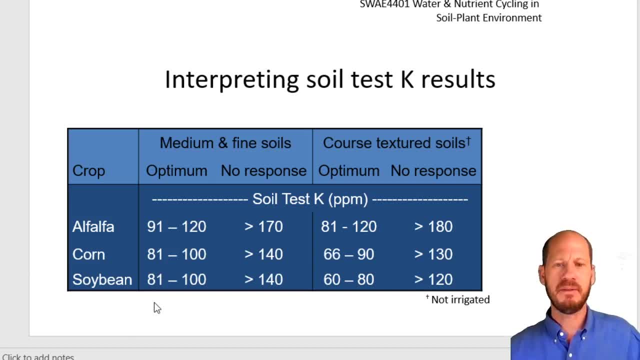 180, you will have a rough idea where your potassium level are. if it's between 100- 180- you are in the good position. if you are beyond that- beyond 180- 200- you are in the good position. if you are beyond that- beyond 180- 200- you. 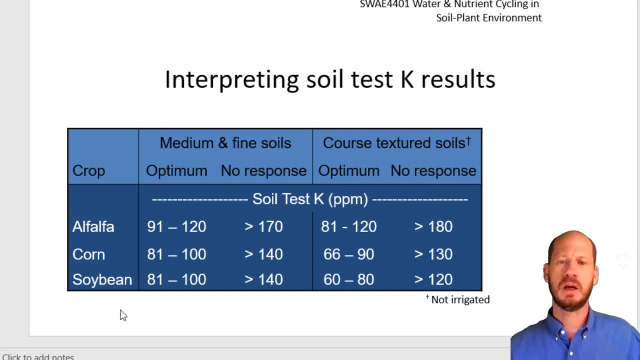 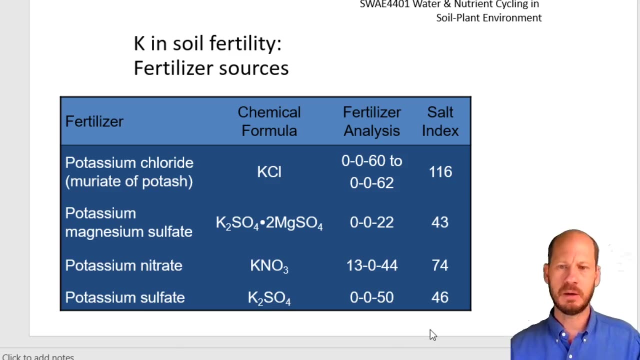 might be willing to deplete, so do safer ranges, and if you are in insufficient levels below 100 ppm, then you might want to apply potassium fertilizer to your crops. yeah, and potassium fertilizer comes in different sorts, and the main ones are: most of them are formarked, but not for attach them on the ground for apportionment. 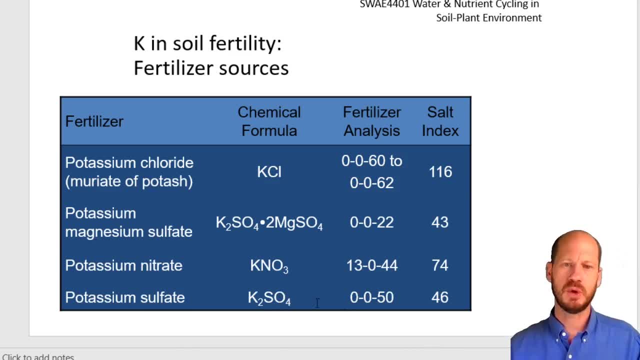 a myriad of Potash, which is Potassium Chloride, Potassium, Magnesium, Sulfate, also Potassium Nitrate, Potassium Sulfate and Potassium Phosphate, is not listed here, but it's also a commonly used fertilizer and it's integral part of the NPK formulas. 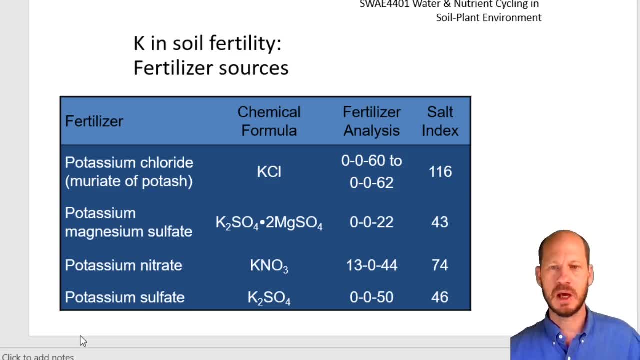 Consider that when you have sufficiency of Potassium, you should choose the NPK formulas that do not contain Potassium or contain a very low amount of Potassium, and when you have deficiency, you should choose the ones which are very high in Potassium. Of course, what I really recommend is that you to base your fertilizer recommendation 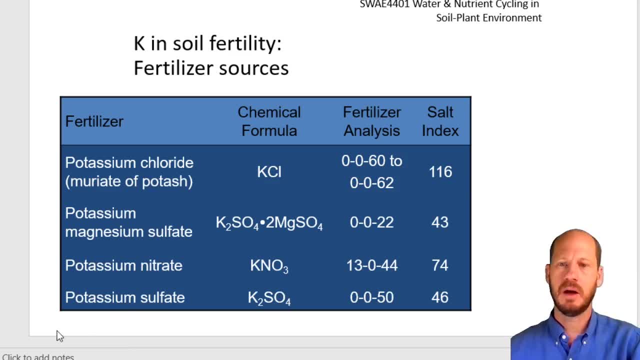 on the Phosphores and the Nitrogen and whatever you add together with the Phosphores and Nitrogen of Potassium, usually you don't have to worry about Potassium too much. If you are adding it as a soluble fertilizer, you will have it enough for the crops. 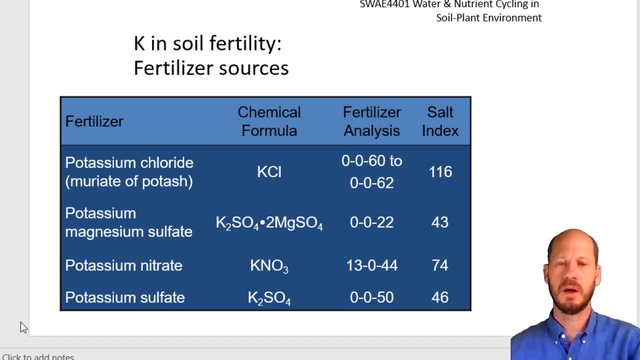 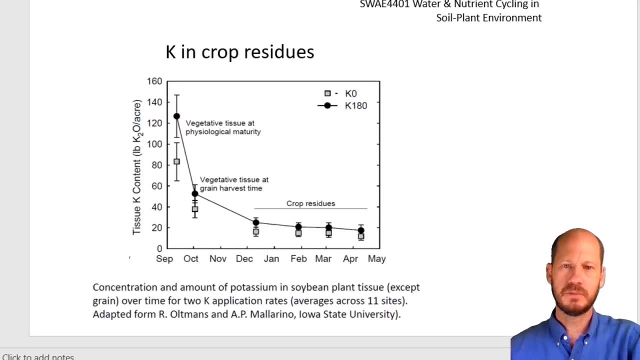 but you should be wary about the excess of Potassium in the soils. usually Okay. this is showing just how the Potassium vanishes from the plant tissue. Potassium is fairly mobile and therefore when the old tissues, the tissues, become old, the concentration of Potassium in these old tissues 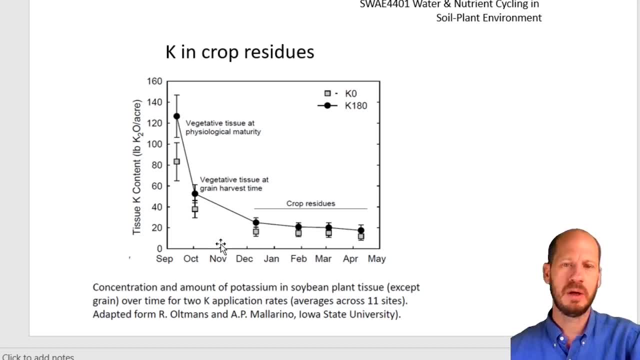 will decrease, will be mobilized to other young leaves and fruits and in the plant residues also, there is a steady decline in supply for the next crop. If you keep the plant residues on the farms, that will be a good source of Potassium also for the next crops. 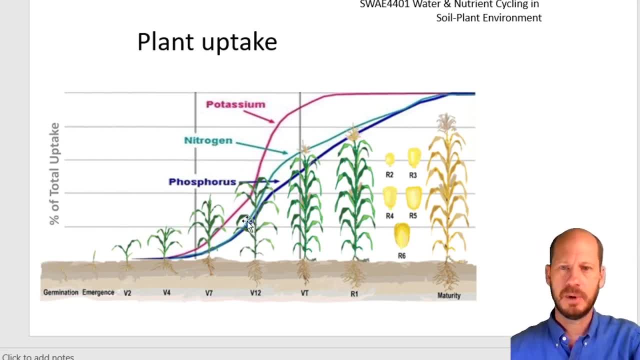 Here is showing that the Potassium uptake by plants is usually very strong on the early stages of the plant growth. If you supply Potassium as a starter, which is usually what's recommended, then the plant will uptake all the Potassium it needs and then it will reuse and redistribute. 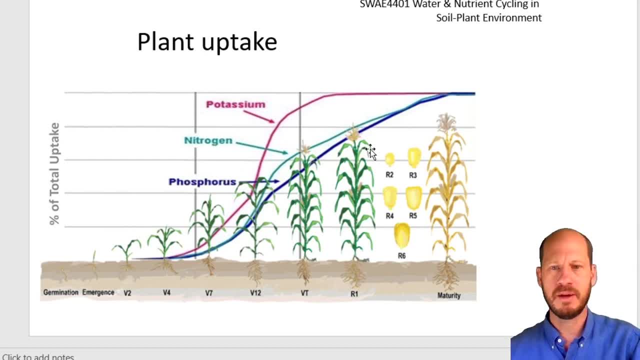 that throughout the season on the plant tissues and you don't have to worry too much because the Potassium that is uptaken can be easily redistributed and will be enough for the full cycle of the crop, Whereas for Nitrogen and Phosphorus there's a more steady uptake and a need of constant 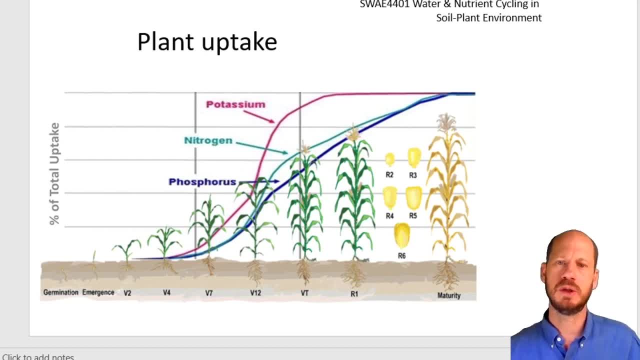 amount and availability on the soil solution Potassium can be easily. if you have a high concentration on the start of the crop, that is enough for supplying for the soil. So you have a good supply of Potassium but you have to worry about the full cycle. 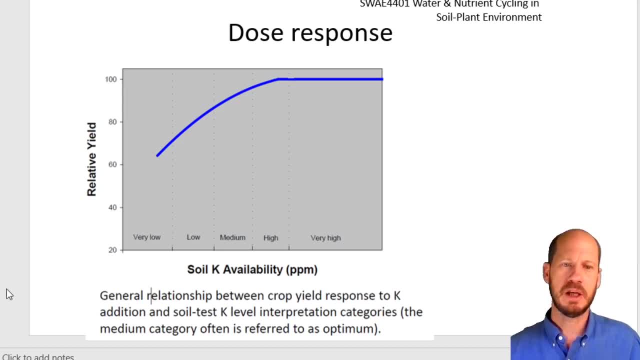 You can have the same type of dose response of fertilizer recommendation that you see for Nitrogen and Phosphorus until you have the sufficiency levels, that is, usually over 100 ppm on the the soluble Potassium in the soil. Regarding the application of Potassium and timing, 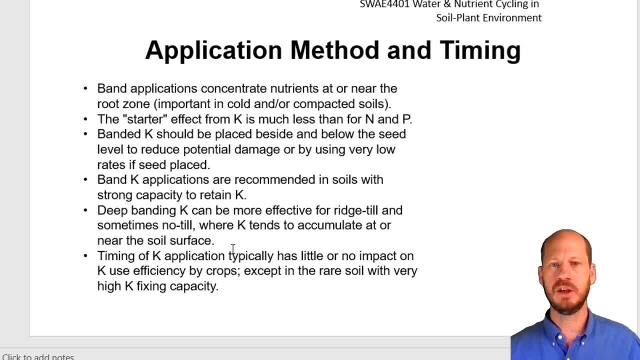 try to use band applications and near the root zone to maximize the efficiency of the potassium fertilizer. always use it as a starter it's, but consider also that when you want to really see the response of the plants, this effect of potassium is much less evident than it is the effect of nitrogen and phosphorus. 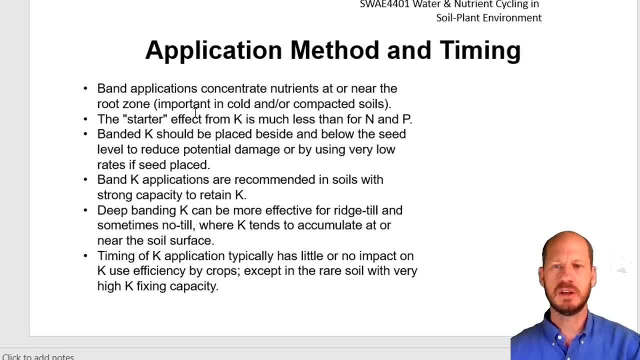 the plant response when you're nitrogen deficient or phosphorus deficient and you apply nitrogen and phosphorus is very, very visible. in the case of potassium is usually less so, so you should not be concerned. just when you do your fertilizer application with nitrogen and potassium, use a formula. 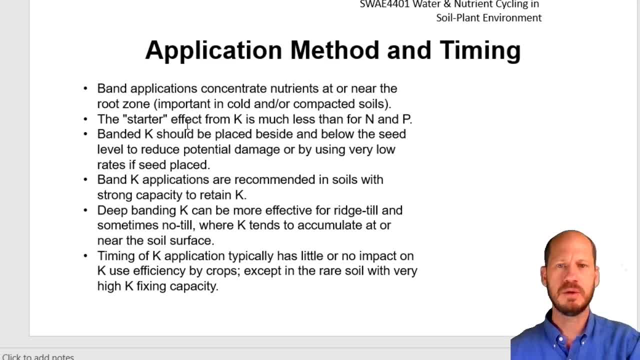 that also contains nitrogen and phosphorus. you use a formula that also contains some amount of potassium, and usually that would be an enough, you know. so when you do it banded K, you should do it below the sea level to maximize the optimized the plant uptake of this potassium. when you 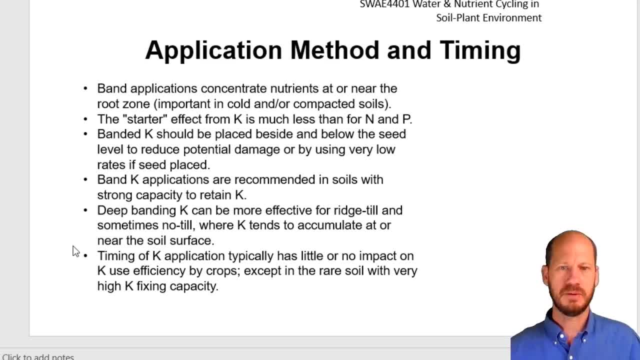 have soils with strong capacity to retain a potassium, you should always try to do the band application near the root zone. the timing normally does not have any impact on potassium use for crops, so ideally you do it in the start of the crops and that will make that you will have no issues. 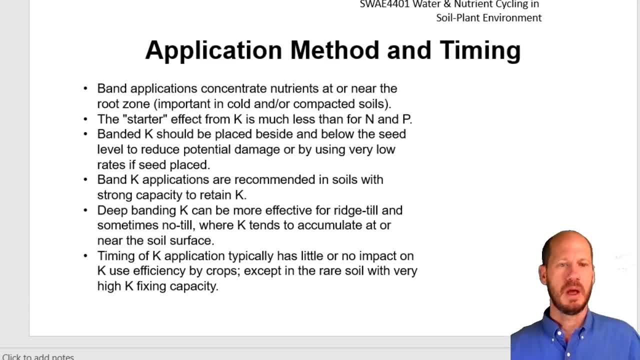 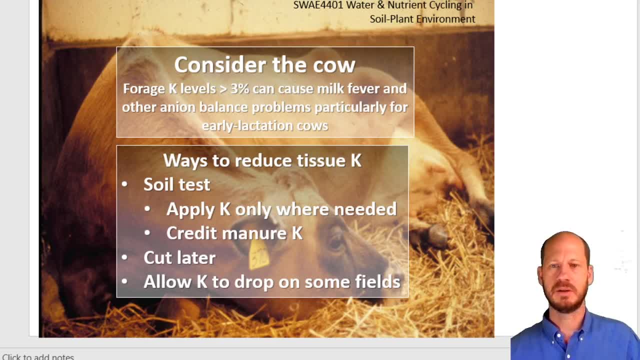 with potassium whatsoever. the main issue of potassium, of course, is when is not when you have deficiency, because if you are, if you have a fertilizer program you you use, usually will have sufficiency of potassium. the main issue for for potassium is the excess of potassium, and this is more and more important when. 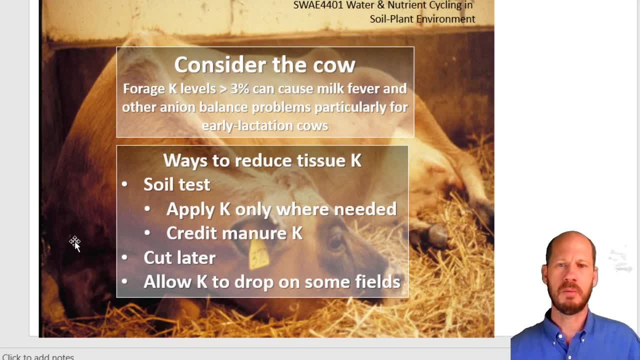 you have. you're using your crop residues for dairy farms, so when you have excess potassium on the plant tissues, you can cause milk fever to the cows. so it's very important to test your soils and make sure you don't have excessive potassium concentration on your soils and if you do have, you need to consider. 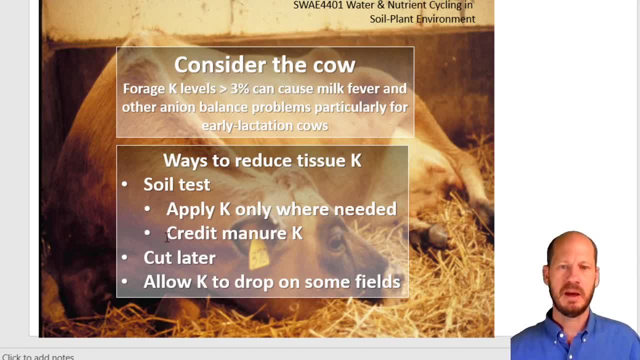 a depletion program, to have to find a way to decrease your potassium levels to acceptable ranges. one of the things you can do in these situations, when you have excess potassium on the soil, is to delay the time you cut your plants. you will have less proteins, so there is a high chance that your plant is not getting enough potassium. 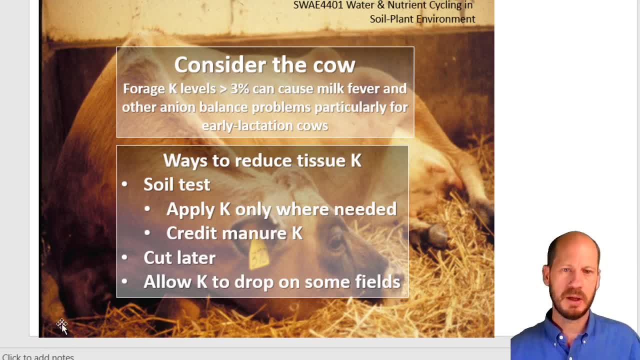 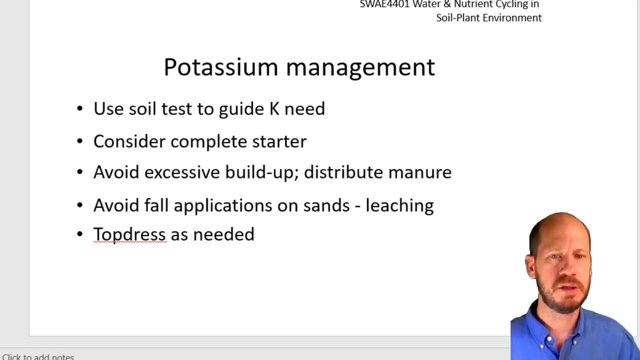 but also you will have less potassium. you know you will increase the fiber content but the potassium will be mobilized and then you will have less potassium on the plant material. all in all, to wrap up the fertilizer recommendation strategy, you should think base your fertilizer recommendation not 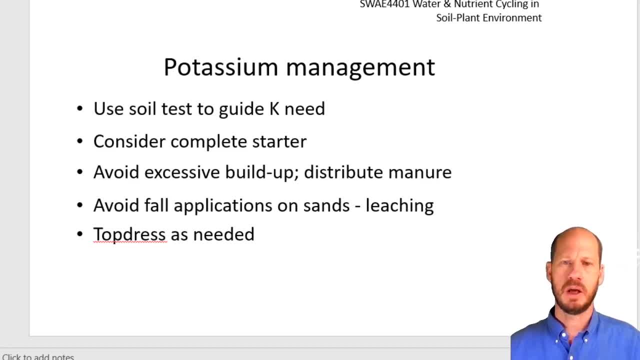 in potassium. base your fertilizer recommendation in phosphorus and nitrogen. it's very hard to balance 3 nutrients on the fertilizer formula. so if you have deficiency, consider a formula that contains potassium and that will be enough, but base your fertilizer recommendation mainly on phosphorous and nitrogen, which are the most problematic nutrients for the nutrition.